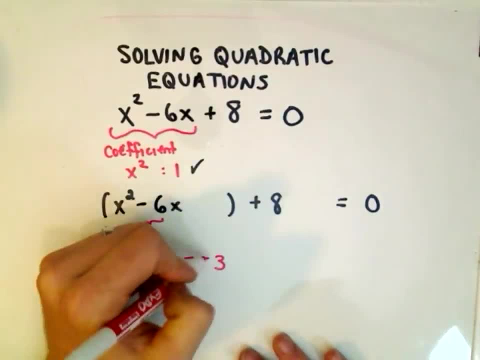 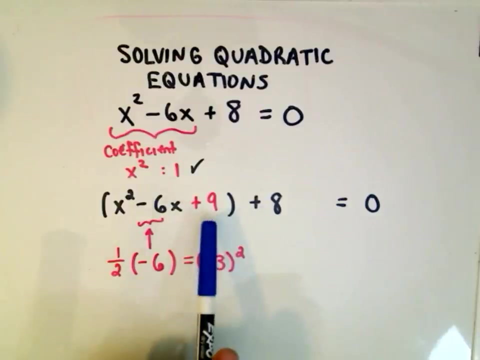 So 1 half of negative, Negative 6 will be negative 3. And then what you do is you square it and then you put that number back inside of there. So if we square it, we'll get positive 9.. Okay, so we've actually just thrown in a brand new number that wasn't there before. 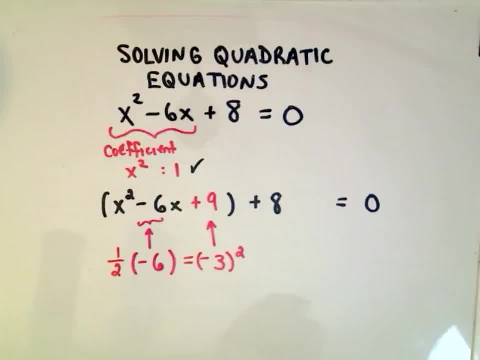 We put in this positive 9 that wasn't there. Well, the way that we can get rid of it in this case is, I mean, basically imagine just getting rid of the parentheses. We would get back the original thing, except our plus. 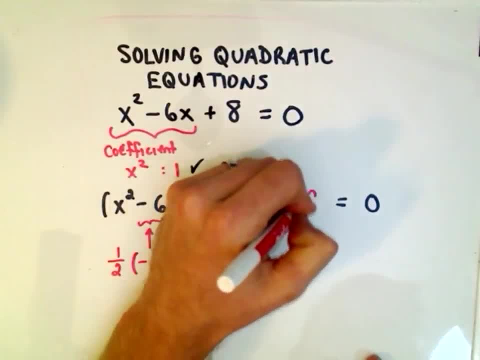 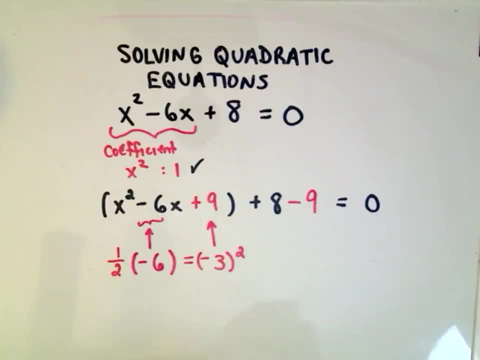 9 would be there. Well, to cancel it out, we're going to subtract 9, okay. Notice, this is all happening on the left side of the equal sign. Okay, so now we just simplify down a little bit more, And the point is you can write this stuff in parentheses as a perfect square. 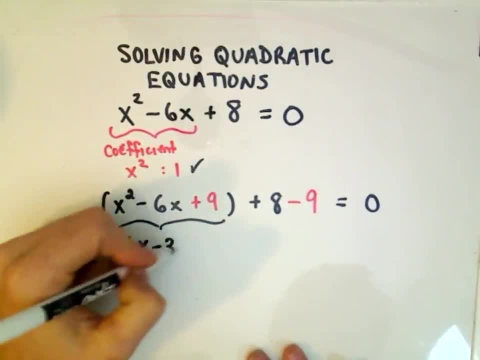 This actually factors now as x minus 3 times x minus 3, okay, And again, if you take Whatever one-half of the coefficient on the x term was, it was a negative 3.. That's what will go inside the parentheses. 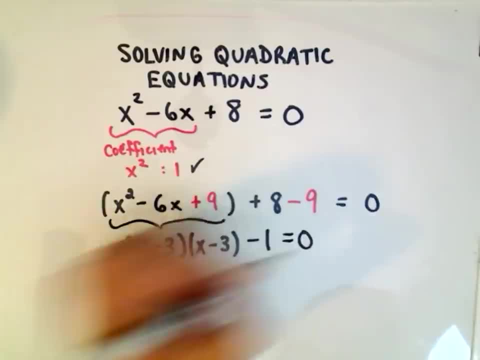 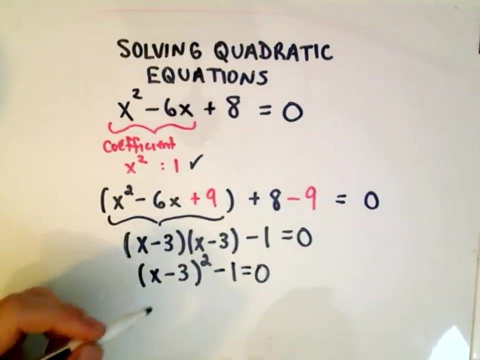 Positive 8 minus 9 is negative. 1, equals 0.. So now we write the first part as x minus 3, squared minus 1, equals 0.. Okay, so again we're trying to solve a quadratic equation here. What we do at this point is you now simply add the 1 to both sides. 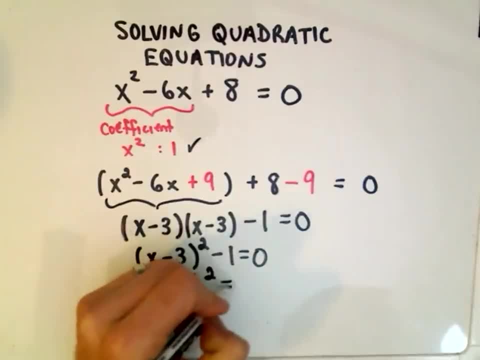 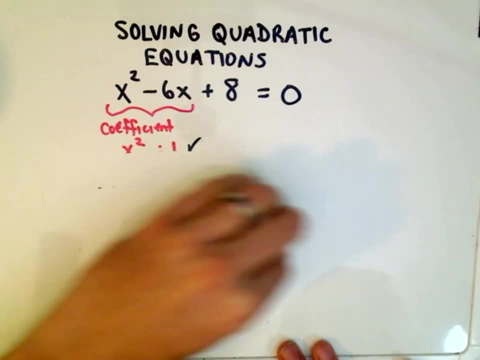 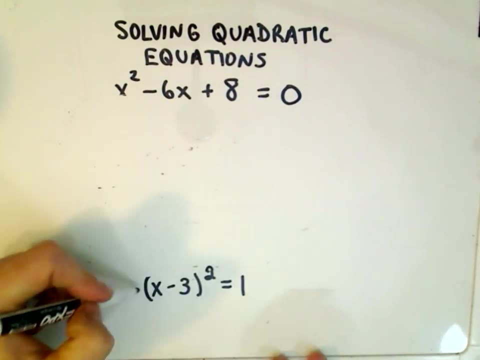 So x minus 3. Squared equals positive 1. And the whole point of solving a quadratic equation by completing the square is getting to the step that we're at right now, Because what we're going to do is we're going to take the square root of both sides. 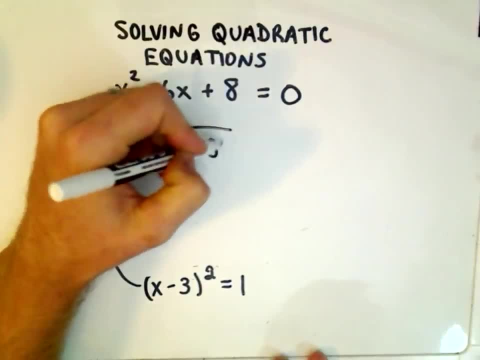 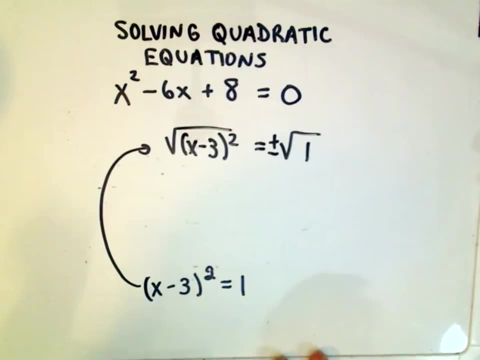 So if we take the square root of both sides, x minus 3 squared equals the square root of the right side. Okay, so once we take square roots, we should put a positive or negative On the left. if you take the square root of a quantity squared, we'll just get the x minus 3.. 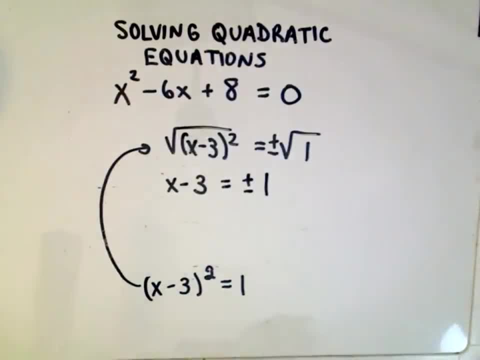 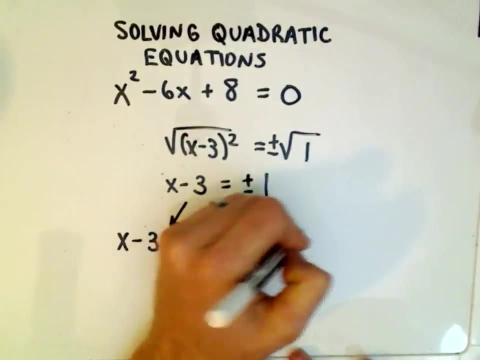 And this will equal either positive or negative 1.. So now we get our two separate equations that we have to solve. One of the equations that we'll have to solve will be: x minus 3 equals positive 1.. And then the other equation we'll have to solve will be: x minus 3 equals negative 1..